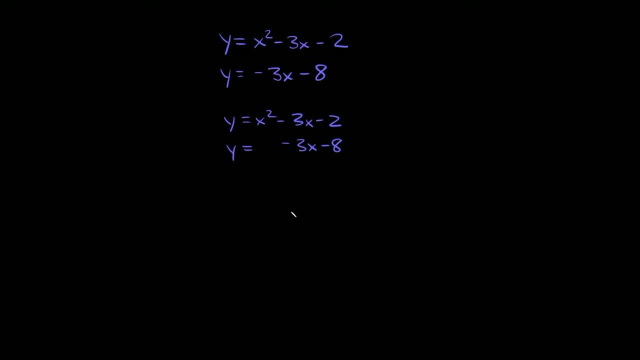 the other just a number, so minus 8, like that. okay, So we're going to subtract this equation and then we're going to do the same thing over here. So we're going to do the equation from the top one. okay, so we're going to subtract this whole thing away. so first of all, y. 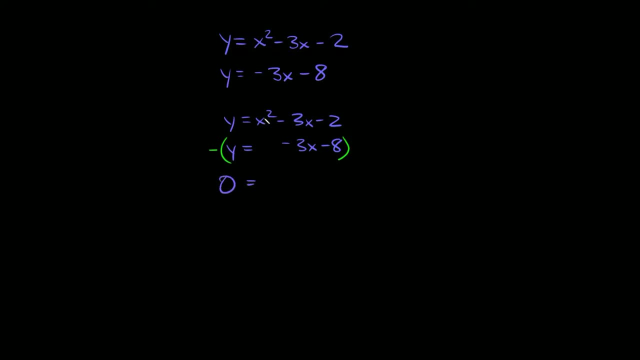 minus y, that's equal to zero. so then that's going to be equal to here: x squared. basically, minus zero is just x squared. and then here, negative 3x minus negative 3x- well, that's the same thing as negative 3x plus 3x, right, and that's equal to zero. all right, so we just have a zero there and then negative. 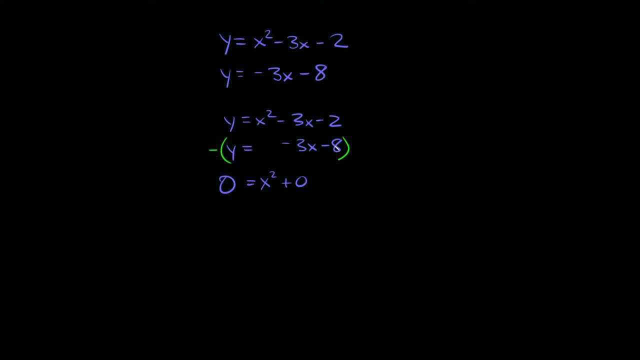 2 minus negative 8. well, again, subtracting a negative is the same thing as adding, right, so negative 2 plus 8 is equal to positive 6, right so plus 6. okay, so then here we get. zero is equal to x squared plus 6. okay, so we're just trying to solve for x now. so the first thing we're going 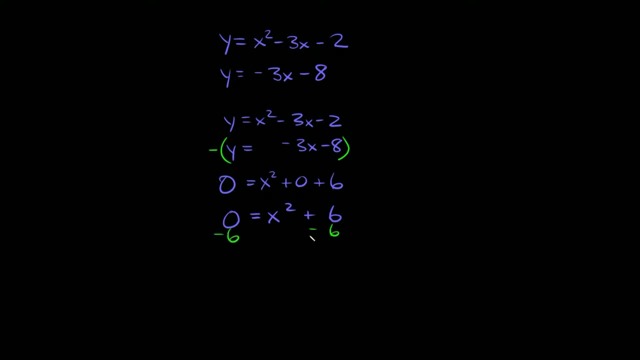 to do is subtract this 6 from this side, and what we do to one side we do to the other, right. so those cancel out, and then here we get zero minus 6, which is negative 6, and that's equal to x squared squared. Okay, so x squared is equal to negative six. Now this is a problem because there's no. 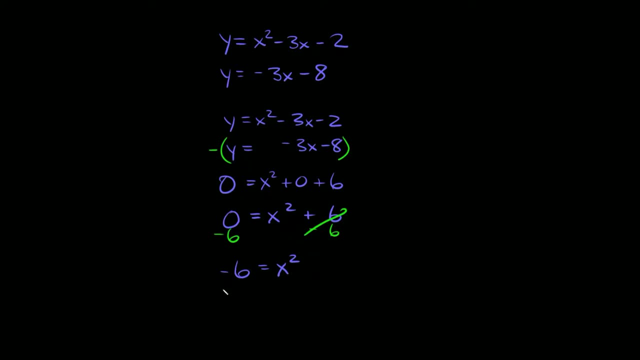 number that you can square that gives you a negative number. Okay, so whenever you get x, squared is equal to a negative number, that means there are no solutions. Okay, because again there's no number you can plug into x and then square it where it would give you a negative number, right? 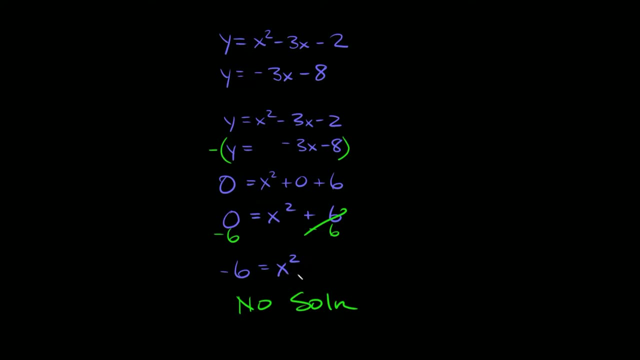 because whenever you square a number, it always gives you a positive number, right? All right, here's the next one. So here we have: y is equal to negative, x squared minus 2x plus 2, and y is equal to 4x plus 2.. Okay, so again, the first thing we're going to do is just subtract one of this. 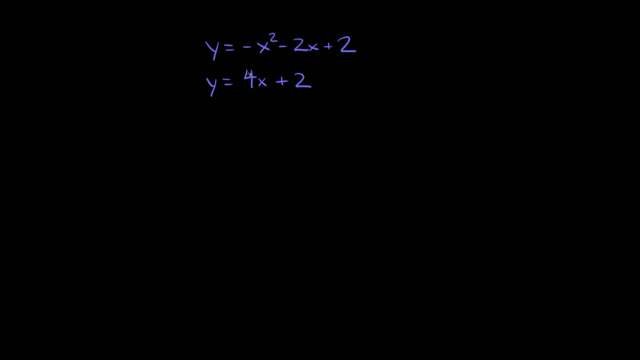 bottom one from this top one. Okay, but before you do that, you always want to line up your terms, right? So I'm just going to actually scoot these over like that. Okay, so now the x terms are lined up and our numbers are lined up, right, So now we can subtract this whole number from the bottom. 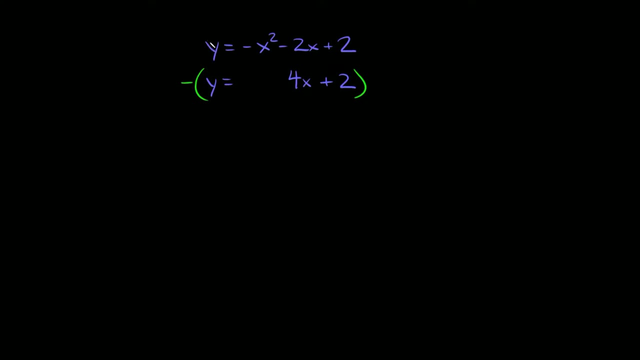 equation from the top one. Okay, so again, first of all, y minus y, that's just equal to zero. Okay, here we have negative x squared minus zero, it's just negative x squared. and then negative 2x minus 4x is equal to negative 6x. and then here, 2 minus 2 is equal to zero. All right, so we don't. 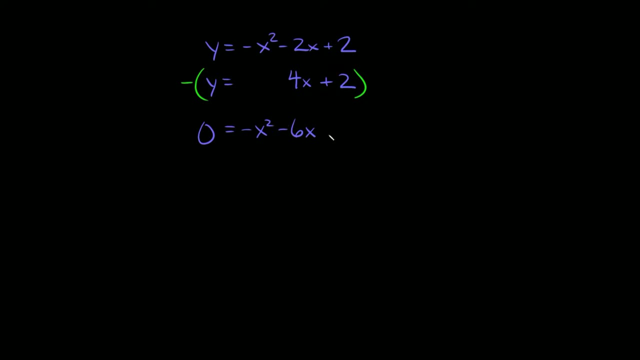 have anything there. So we get zero is equal to negative x squared minus 6x. Now we just need to factor this. Okay, so the first thing we're going to do is we're going to factor this. So we're going to do is factor out a negative x from each term, Right? so we're going to get zero is equal to. 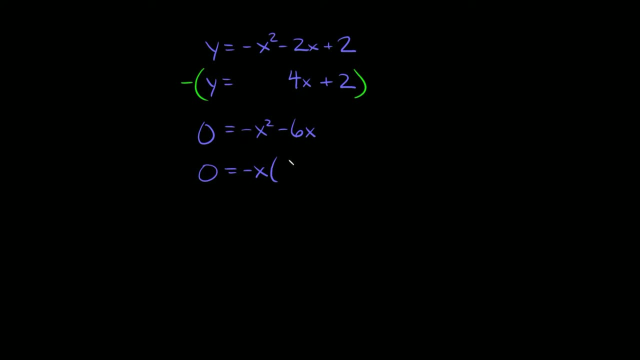 factoring out a negative x Inside the parentheses, we're just going to be left with an x and then a minus 6.. Okay, so, now that we've broken this all the way down, you can see we're left with two factors. right, We have this negative x right there, and then we also have what's in parentheses, this x. 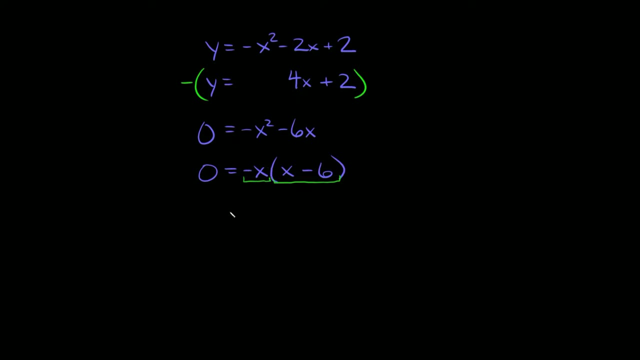 minus 6.. So then you just want to set each of these equal to zero. So we're going to say negative x is equal to zero and x minus 6. Is equal to zero. Okay, because we just have to solve for the x's and the way you do that again. 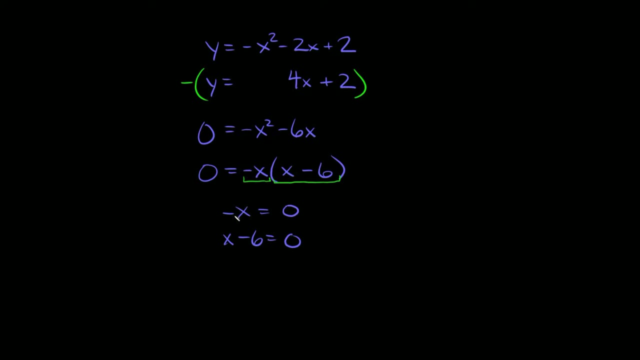 is just setting each one equal to zero. So here for this first one, negative x is equal to zero. Well, x would have to be equal to zero. and then down here, x minus 6 is equal to zero. X would have to be equal to positive 6.. Right, because 6 minus 6 is equal to zero. Right, so then we get: x is equal to. 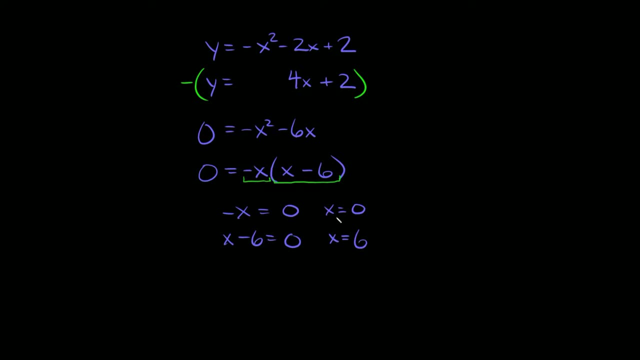 positive: 6. Right, so, as you can see, we got two answers right: X is equal to zero and x is equal to 6.. So now we have to find the y values that they're paired up with, And to do that, all you have to do. 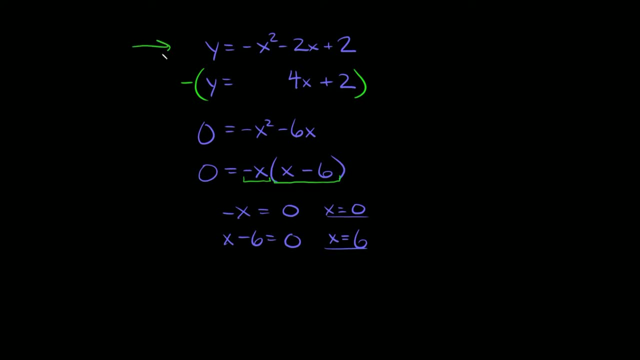 is plug in these two back into either one of these original equations, And I'm going to use this one right here because it looks like it's a lot easier to work with than this top one up here. So it's: y is equal to 4x plus 2.. Right, so y is equal to 4.. But for our x, for this first one, let's plug in a. 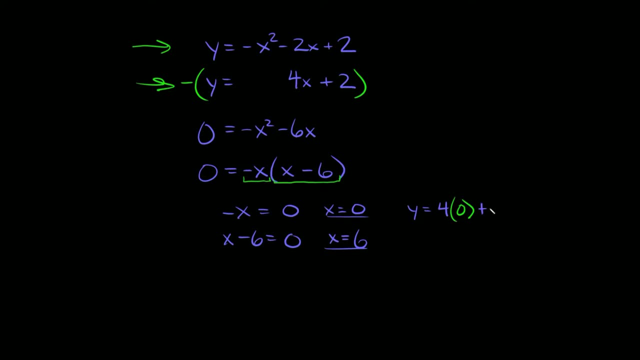 zero. So we're going to plug in a zero right here, Right, and then we have positive x plus 2.. Right, and then we have plus 2.. 4 times 0 is 0.. 0 plus 2 is equal to 2.. Okay, and then for this other one. 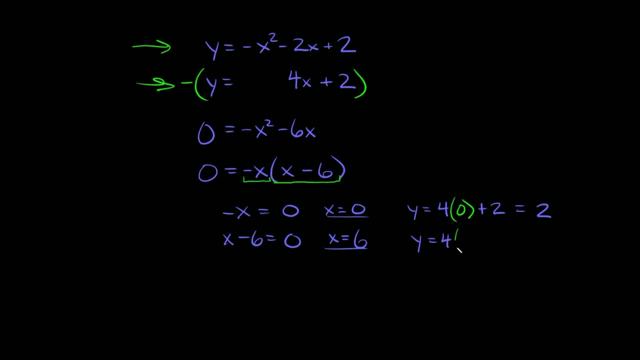 we're going to plug in a 6. So y is equal to 4 times 6 plus 2.. So then, 24 plus 2 is equal to 26.. Okay, so then your solution is going to be a coordinate or an ordered pair. So the first. 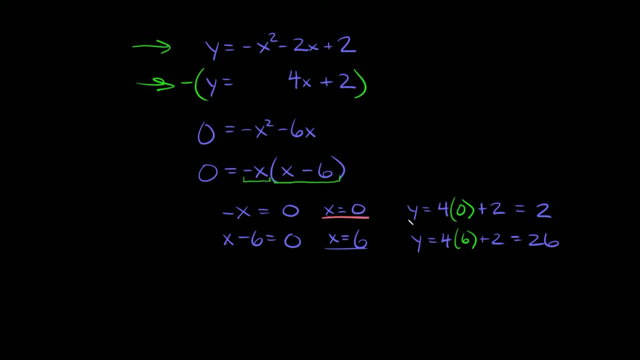 ordered pair that we have is going to be 0 and y is equal to 2.. Right, so our first solution is at 0.. Positive 2.. And then our second solution is at 6 comma 26.. Right, 6 comma 26.. Okay, so there's your. 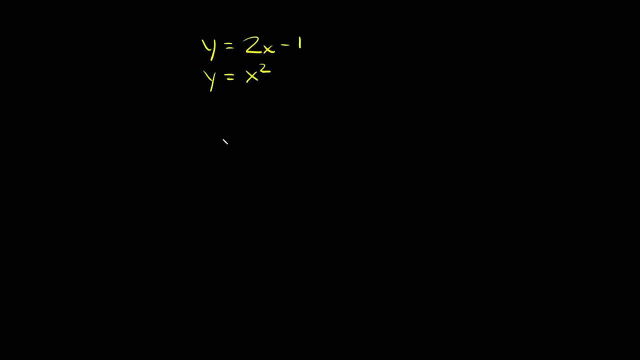 two solutions to this system of equations. Okay, now, the last one we have here is: y is equal to 2x minus 1, and y is equal to x squared. So, again, we're going to subtract these, but we have to line them up first. Right? so the first one, we're going to write it as y is equal to. Now we don't have an. 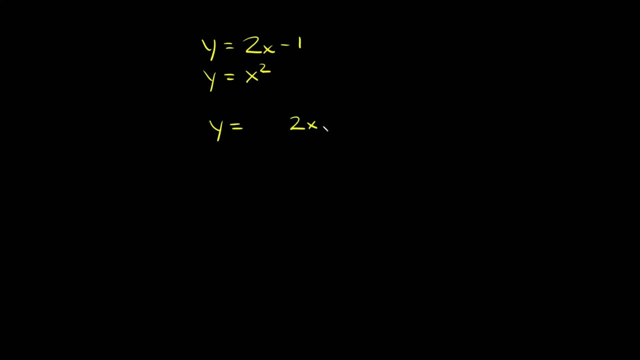 squared term on top. So I'm going to move everything to the side over here. So 2x minus 1, like that. And then the bottom one. we're going to write it as y is equal to x squared, like that. Okay, and remember, we're subtracting away this bottom one, Right? so again, first of all y. 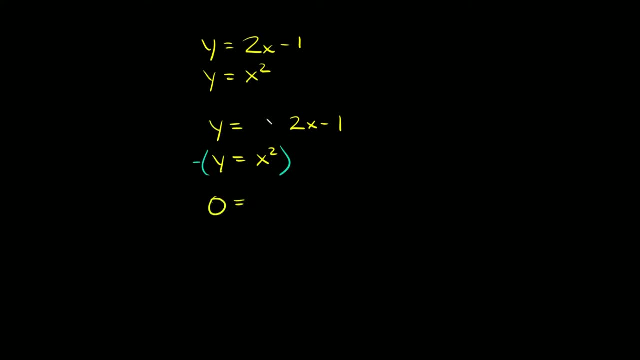 minus y, that's equal to 0.. So then this is equal to: let's see: 0 minus x squared is equal to just negative x squared. And then 2x minus nothing is just equal to 2x. So plus 2x. And negative 1 minus nothing is just equal to negative 1.. So minus 1.. Okay, cool, So now. 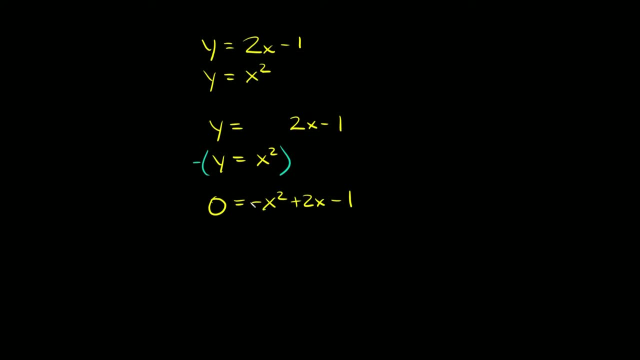 we just have to factor this, And one thing I'm going to do here is I don't like this negative symbol at the very front over here in front of the x squared. So to get rid of that, I'm going to divide this whole side by negative 1.. Right, because that's going to flip the sign on everything. 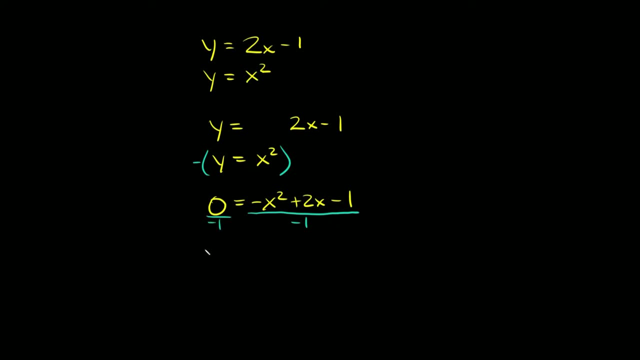 And remember: whatever we do to one side, we do to the other Right. so we'll do the same thing over here. So 0 divided by negative 1, that's equal to just 0.. So that's equal to negative x squared divided by negative 1 is positive x squared Positive: 2x. 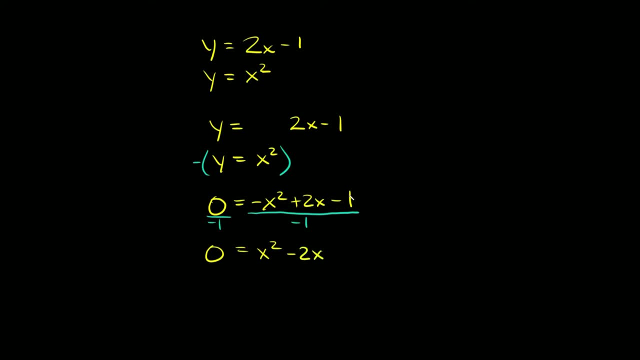 divided by negative 1 is equal to negative 2x, And negative 1 divided by negative 1 is positive 1.. Okay, so now this is a little cleaner to work with Right. so x squared minus 2x plus 1.. So let's factor.